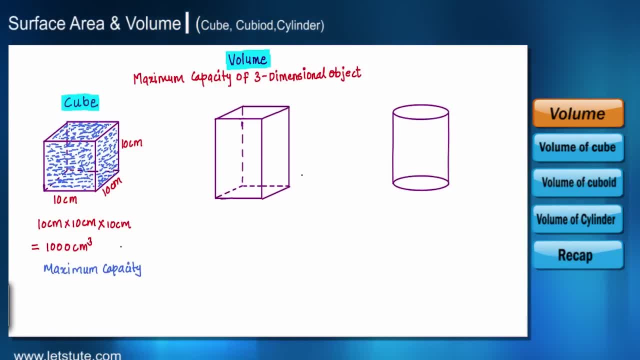 terms of liters, and 1000 centimeter cube equals 1 liters. that means we can say that the volume of a cubicle container having 10 centimeter of length is 1000 centimeter cube or 1 liter. now let's try to write the general form of equation. 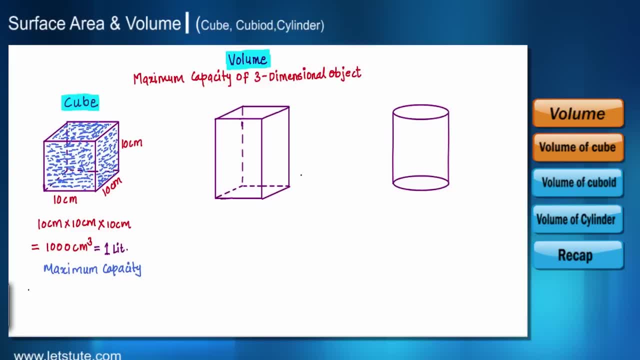 for the volume of any kind of cubicle shape. so if a cubicle container is having length, L centimeter, then the area of base will be squared and we can write it as L squared. and height is also L, so we just multiply the area of base, that is. 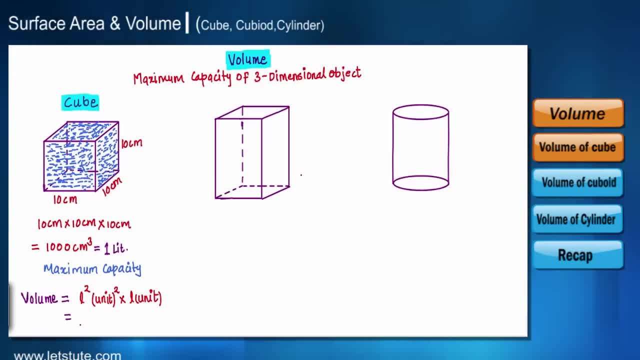 L square into the height L and it will give us L cubed. so the general form of volume of a cube is L cubed, unit cubed. let's try to pour water in the second container, which has length of 10 centimeter, depth, 15 centimeter and height. 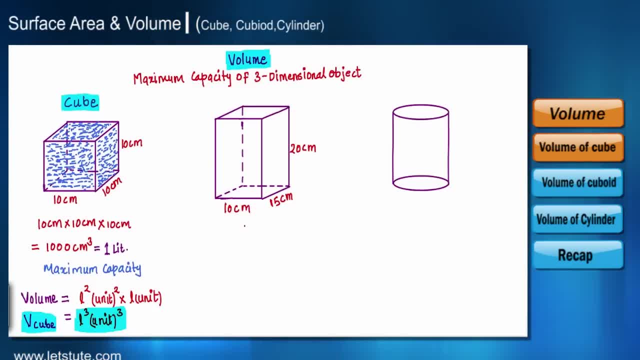 13 centimeter. now, all the dimensions are of different lengths and reality and the first case they all wear same. so if any of the dimension is different, then such kind of shape is called as cuboid and many call it as rectangular prism. so can you tell me how much volume of water this container can have? the 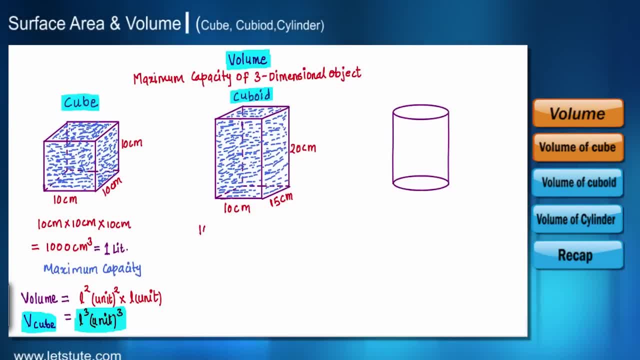 total poured water is the area of base, that is 10 centimeter, into 15 centimeter, 15cm into the height of the container, that is 20cm and it will give us 3000cm3. So we can say that the volume of this shape is 3000cm3 or 3L. 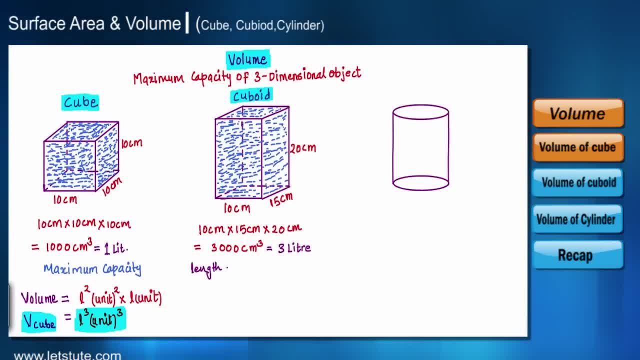 So let's try to generalize it. Let's take length as L, breadth as B and height as H, because all the dimensions are different, so we are using different alphabets. The bottom surface is rectangular, so the area of rectangle is LxB. 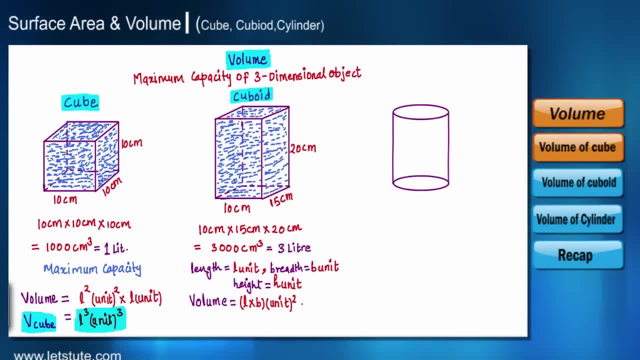 By multiplying the area of base into the height, that is, H, we will get the volume of cuboid. So the volume of cuboid in general terms is LxBxH unit cubed. We can notice one thing: that in such uniform shapes, by just multiplying the area of base, 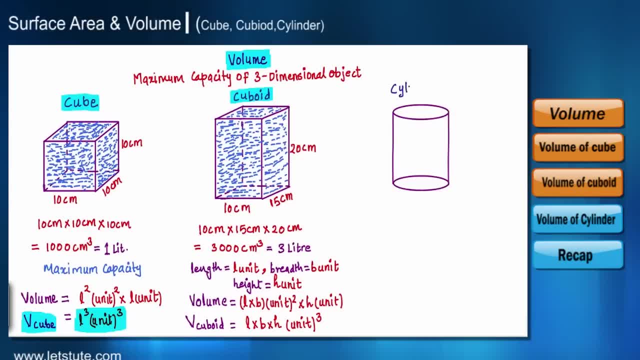 into height, we get the volume. And now we are having one more three dimensional shape, a right circular cylinder. If you look at the base of the right circular cylinder, then the base is circular and the area of any circle with radius r is pi? r squared. 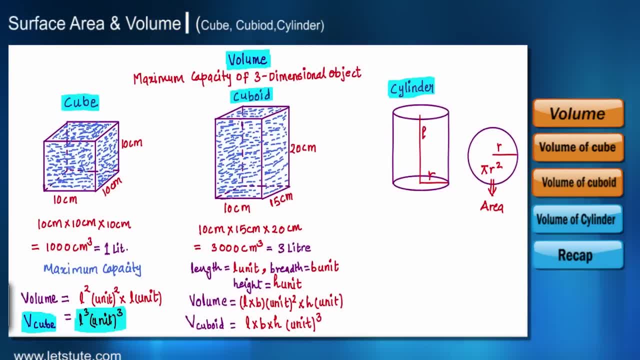 So if you multiply the area of circle to the height, then we will get the volume of right circular cylinder. So first of all we will write the generalization, We will write the general expression for the volume of right circular cylinder, and then we will solve a problem on this. 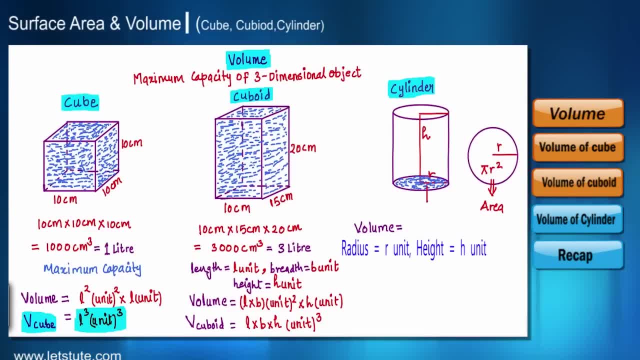 Let's take radius r unit and height H unit. So accordingly, area of base will be pi r squared unit squared into H unit and the volume of cylinder will be pi r squared H unit cubed. So let's solve a problem on this. Suppose a right circular cylinder having radius r 5 centimeter. 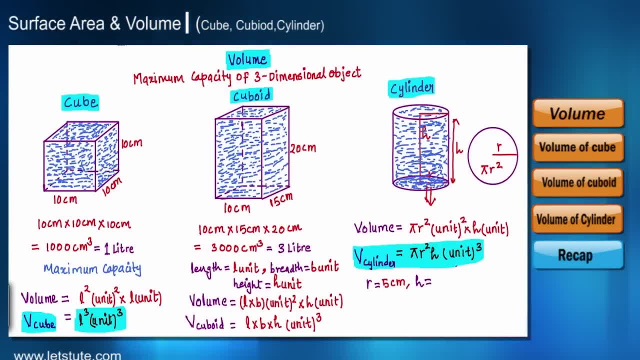 5 centimeter and height of 20 centimeter, then what would be the volume of this cylinder? So by applying formula we get 1570 centimeter cubed or we can say that 1.57 liters. So far we learn about the volume of cube, cuboid and cylinder. 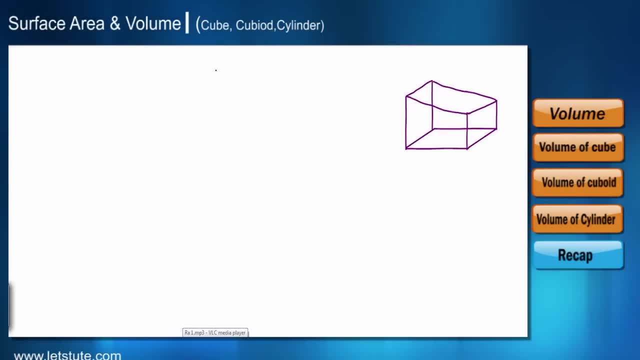 These were the standard shapes, but some of the times we can have uneven shapes like this. So can we find out the volume of this? This three dimensional shape is having length 10 centimeter, breadth, 8 centimeter and in this case, there are two heights. 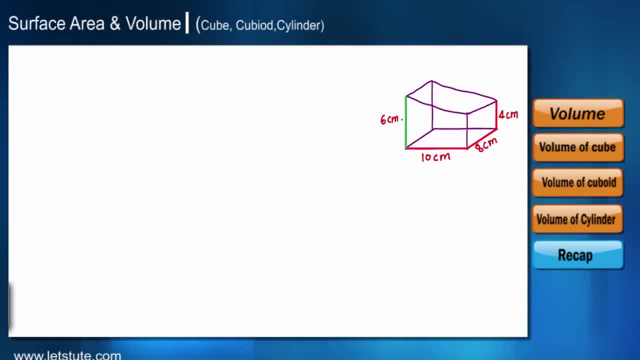 One is 4 centimeter and another one is 6 centimeter And we have to find out volume of this shape. How to go about it? First of all, we have to break it into two parts and we will find volume of each part. 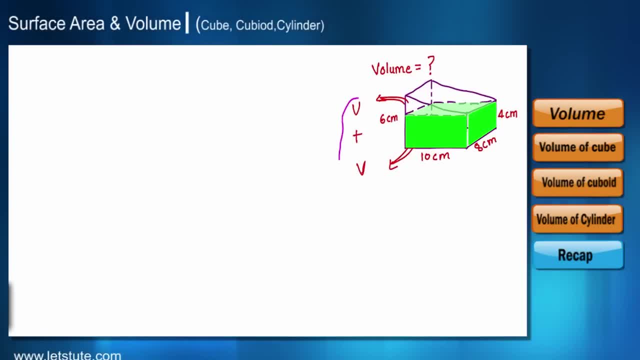 separately. Okay, Add them up to get the volume of original shape. After separating out at the height of 4 centimeter, we got two shapes. So let's start with the bottom part, which is a cuboid with length, 10 centimeter breadth.